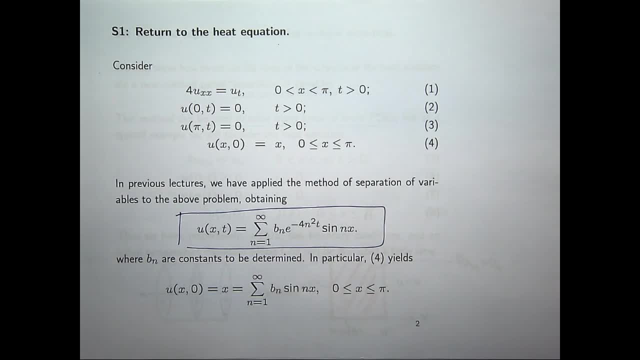 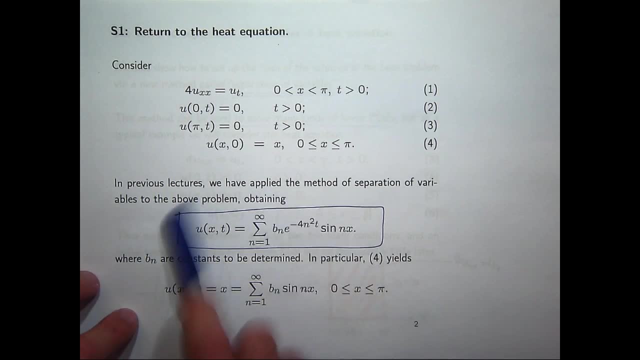 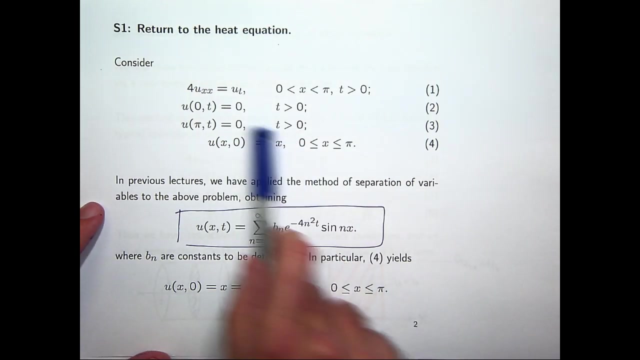 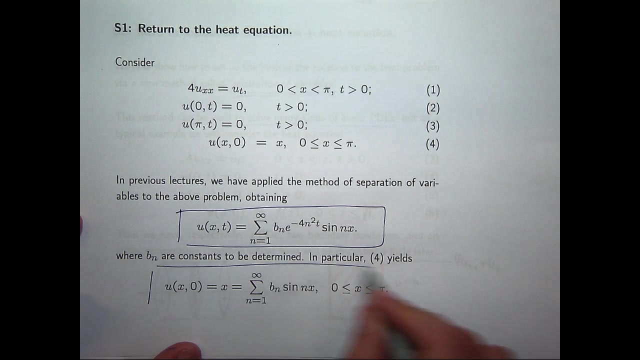 Okay, If you can determine the constants b sub n, then you've solved the whole problem. Now, to get to here, we used these three equations. If you introduce the initial temperature condition just by going in here and putting in t equals 0 and setting it equal to x, then this new 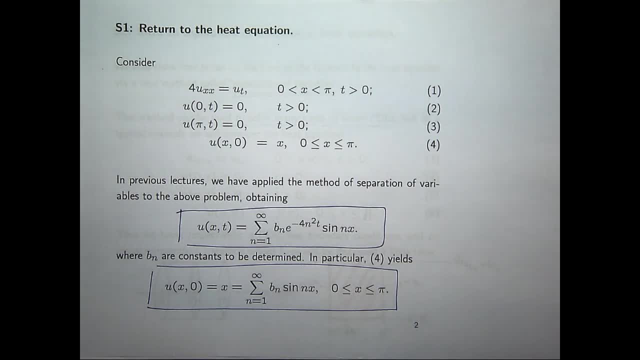 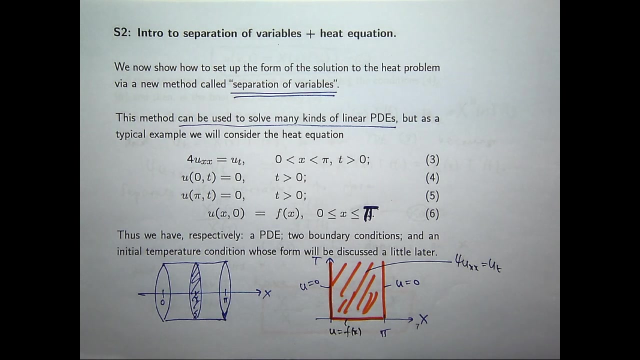 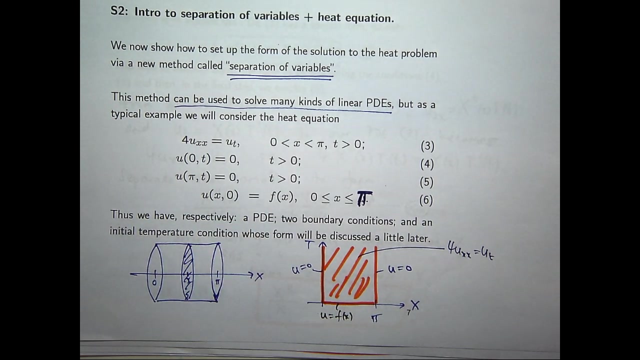 equation gives us the power to compute the b sub n's. Okay, So just to refresh your memory, I'm going to quickly go through the method. So in our, the problem that we'll solve is when f of x equals x here. So you've got a bar in this. 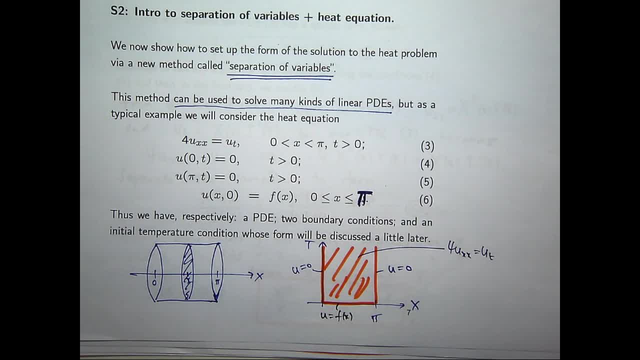 case it's of length pi, which is a little bit unrealistic, But it means the working is a bit neater. U represents the temperature at any point along the bar x and time t. You have some boundary conditions that tell you the temperature is 0 at the ends of the bar And this function. 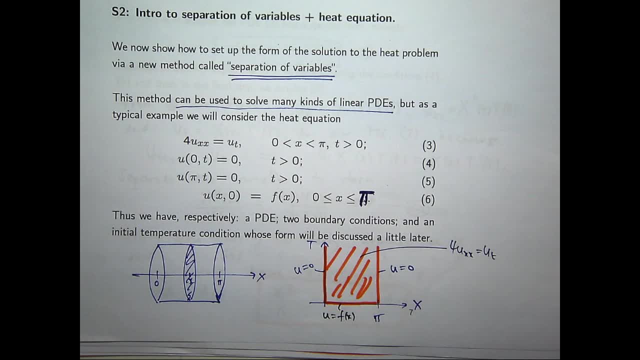 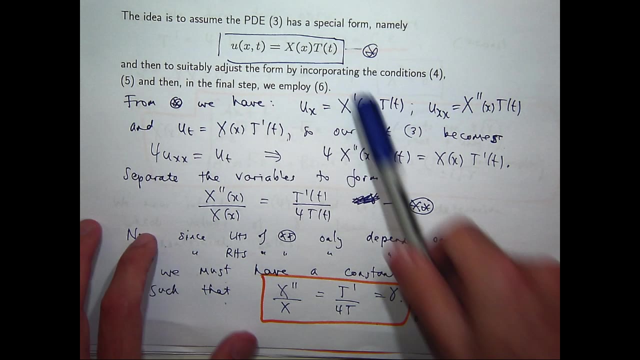 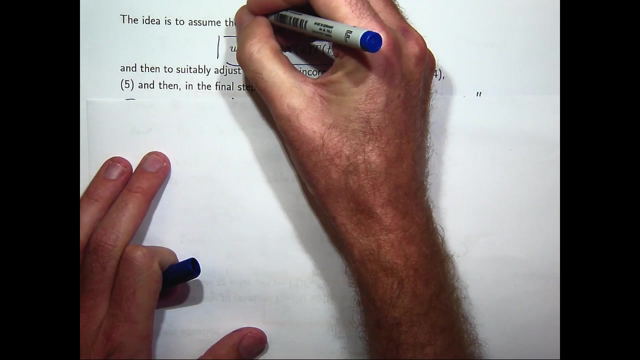 here. this function here is known as an initial temperature, which gives you the you know at any point along the bar. Okay, Okay, At time t equals 0, you have some knowledge of the temperature. So the idea is to assume the PDE or the solution, if you like, to. the PDE has a special form. 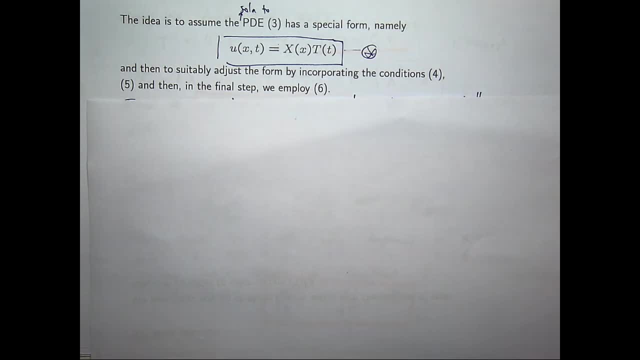 The temperature is a function of position- big X of little x Times- a function of time- big T of little t- And then what you do is you adjust that form by incorporating the boundary conditions and right at the end you employ the initial temperature. 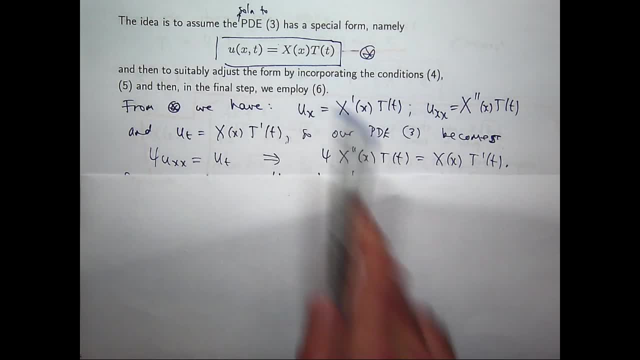 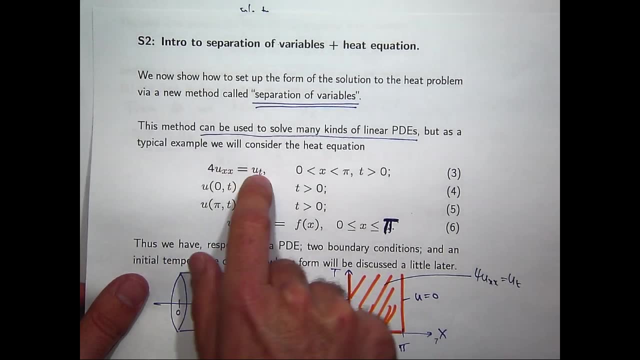 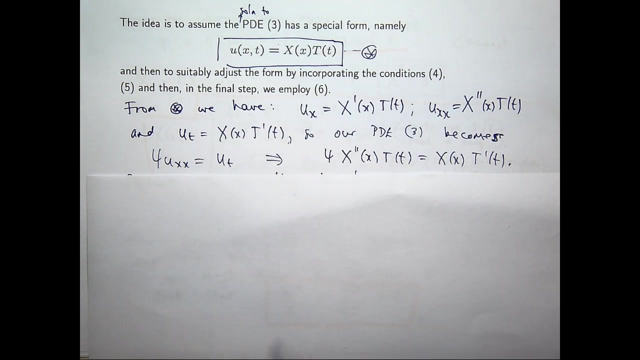 Okay, So with this format. what you usually do with these problems is calculate the derivatives in your PDE. Here I've got u sub xx and u sub t, So you want to take this format, You want to take this form and calculate the partials. 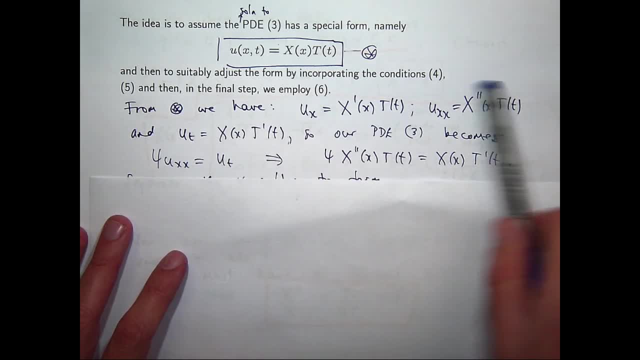 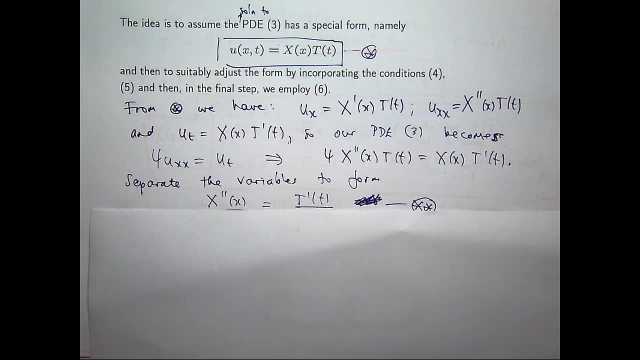 And then substitute: okay, So you would. so here would go here, and here would go here. So you get this set up. Now what you can do is separate the variables, And our aim here is to form two ordinary differential equations that we know how to solve. 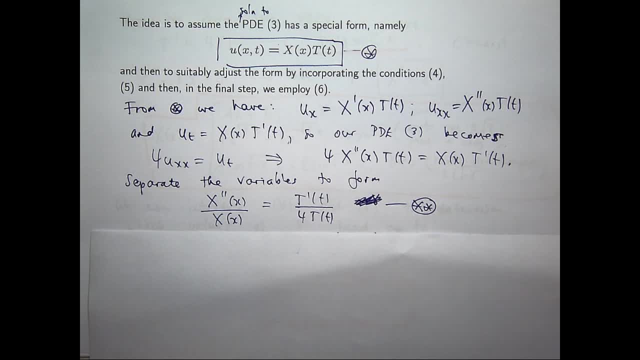 Okay, Now You can see. the left hand side of this relationship only depends on position- little x- Whereas the right hand side only depends on time- little t. So if you vary little x, you would expect this side to vary, But this side can't vary because it doesn't depend on little x. 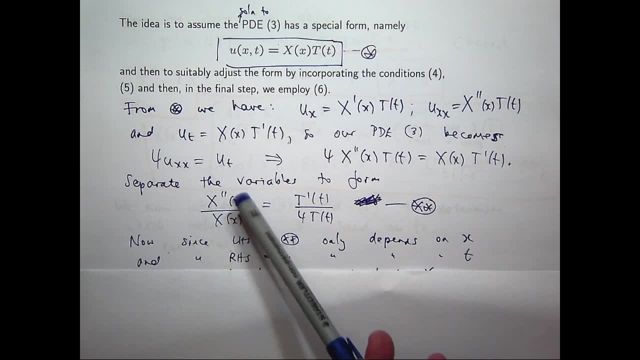 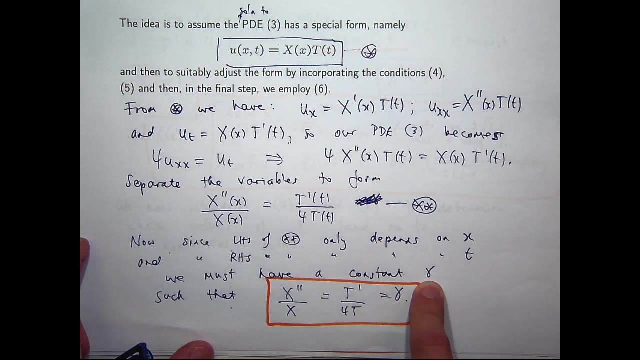 If you vary little t, you would expect this side to vary, But this side can't vary because it doesn't depend on little t, Right? So this format, Okay, That gives us the existence of a special constant, say gamma, called a separation constant. 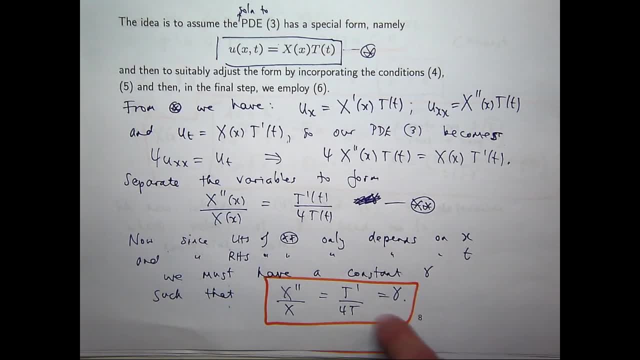 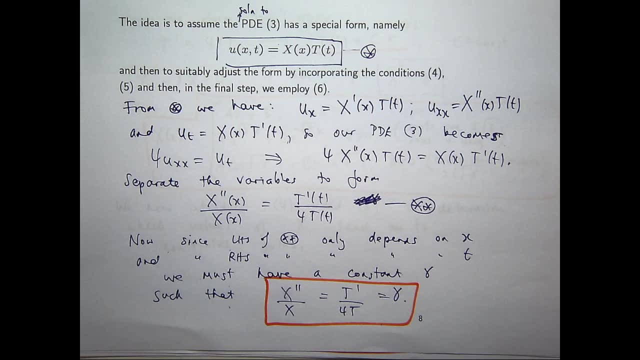 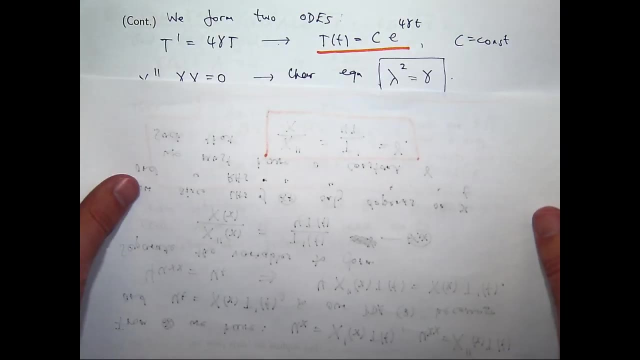 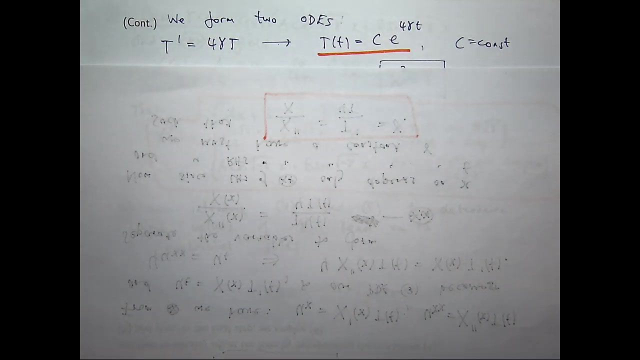 We can set these equal to gamma. So this really now, is the key to forming two ODEs involving that gamma and then solving them. Okay, So if you rearrange these, you'll get two ODEs. The first one In this case it's a first order problem, which can just be. you can just write down the answer. 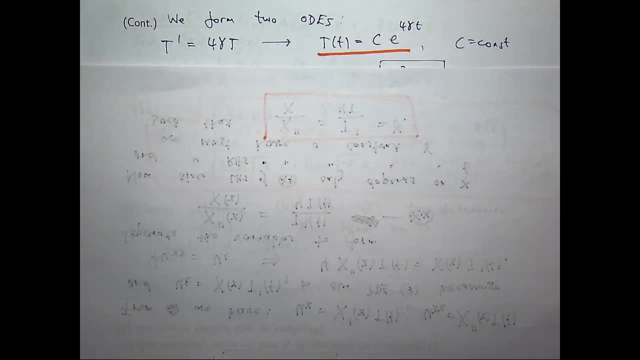 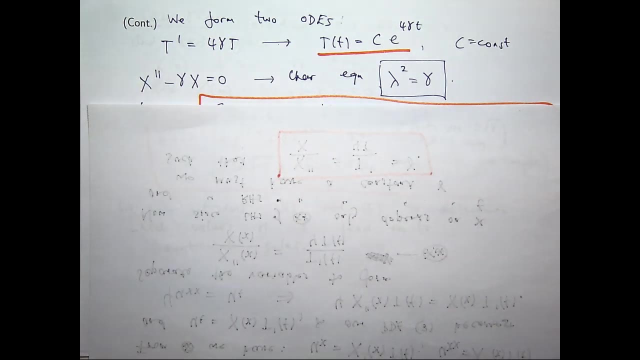 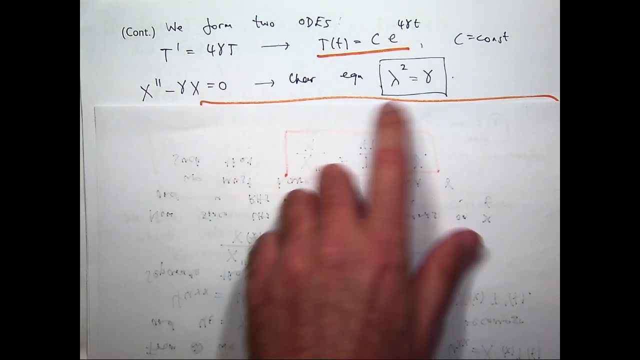 It involves an exponential, And the second one's a little trickier. You've got a second order linear homogeneous problem. Now, usually when we solve these kind of problems, we can solve these problems a number of different ways, But One of the most effective ways to write down the associated characteristic equation- 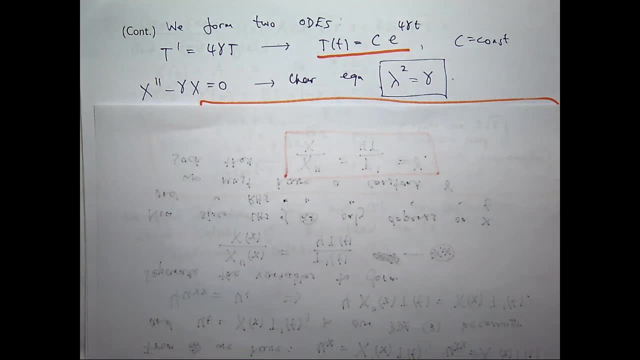 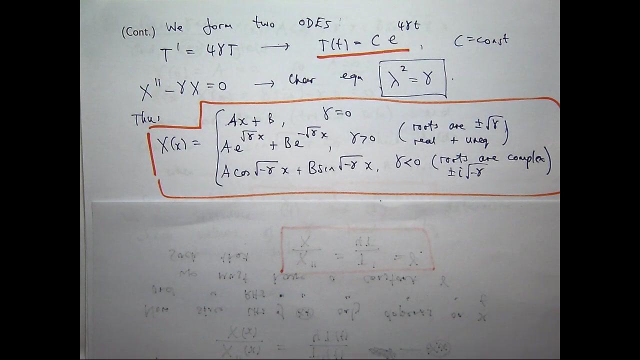 And then look at the roots. Okay, So this is a reasonably simple equation to deal with, But we don't know whether gamma's positive, negative or zero. And that's the next step of our analysis. All right, There are three cases to discuss. 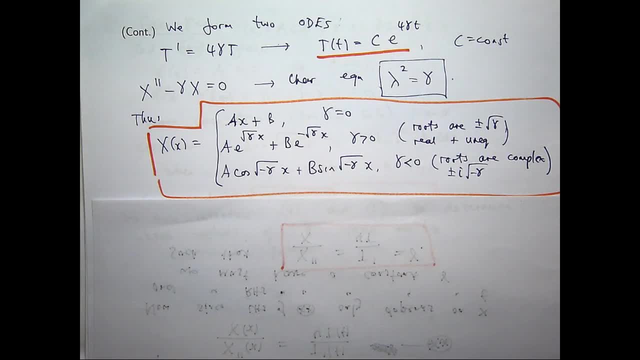 Let's just choose the simplest case, When gamma equals zero. Well, I mean, you can actually solve this problem directly When gamma equals zero Just by integrating, Or you can think of it as the characteristic equation: having real and equal roots, You get AX plus B. 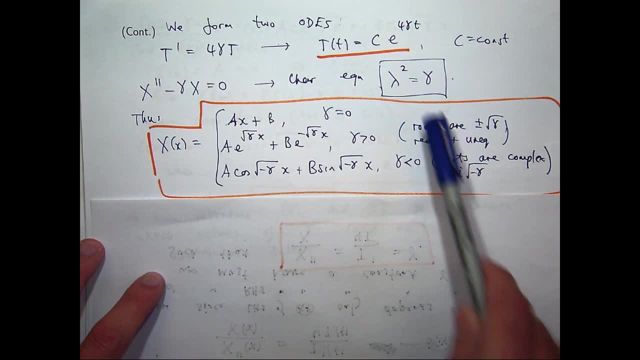 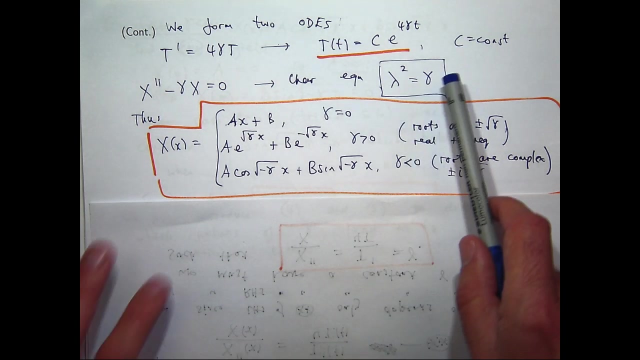 Where A and B are constants, In the case where gamma's positive. well, if I solve that, I'll get roots that are real and unequal. We just form a linear combination of exponential functions, And the last case is when gamma's negative. So 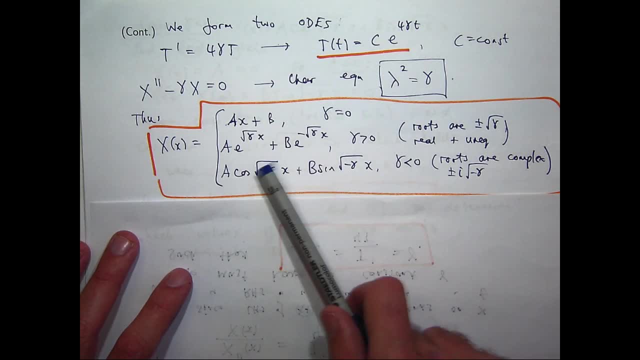 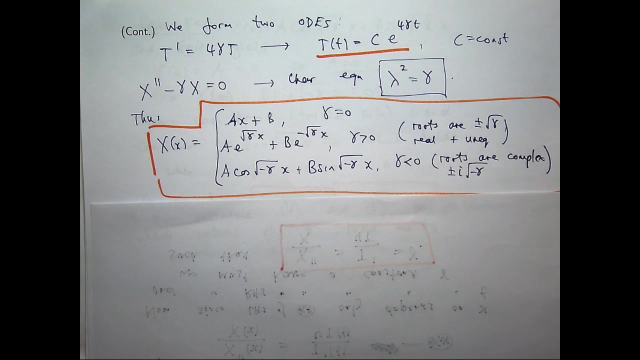 Um, You know, It's just complex roots. And then it's just complex roots with zero real part. In this case it's just a linear combination of sine and cosine. So these are the three forms of this potential solution, And what we do is we try to determine the cases that give you a non-trivial solution. 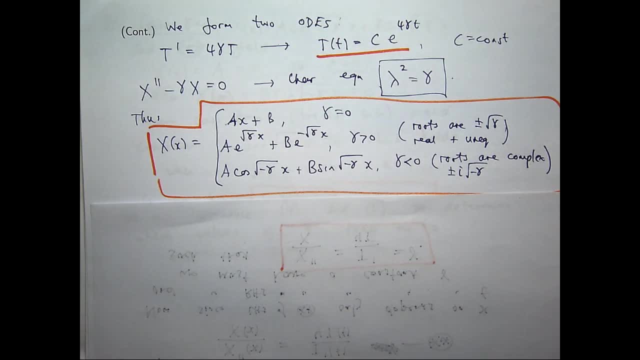 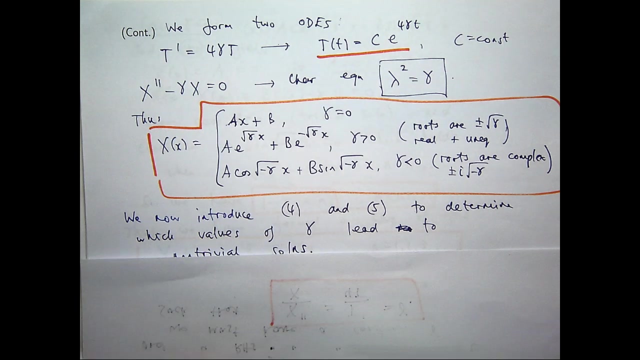 A non-zero solution. Okay, They're the ones we're interested in The non-zero solution case. Okay, So let's introduce the boundary conditions here and here And we'll try to determine which values of gamma give us non-trivial solutions. 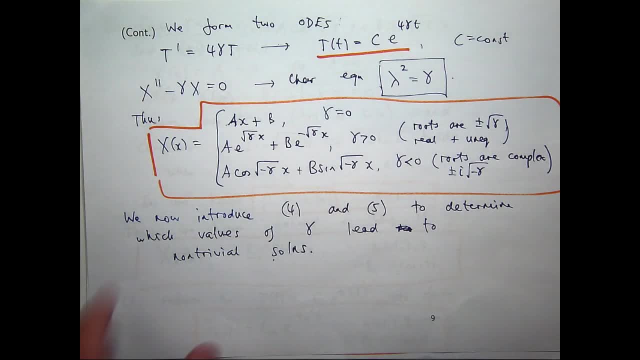 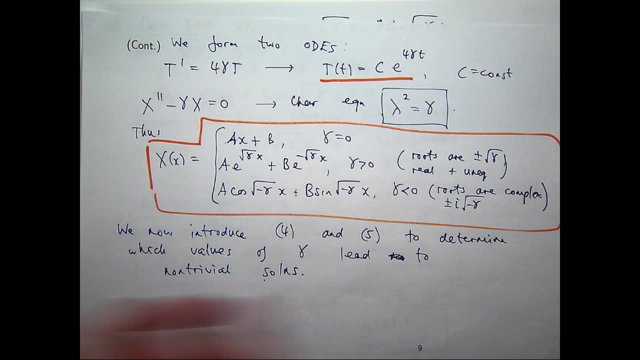 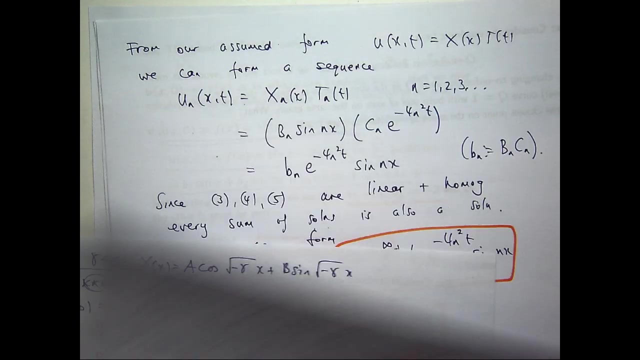 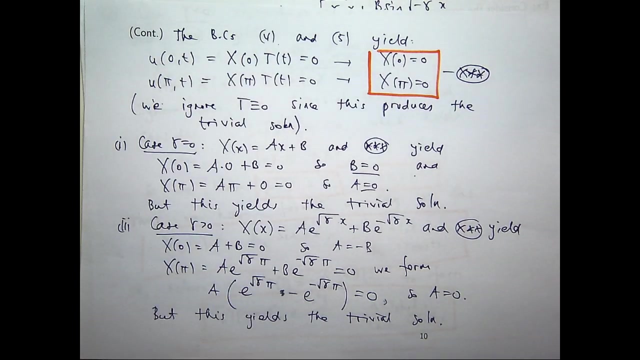 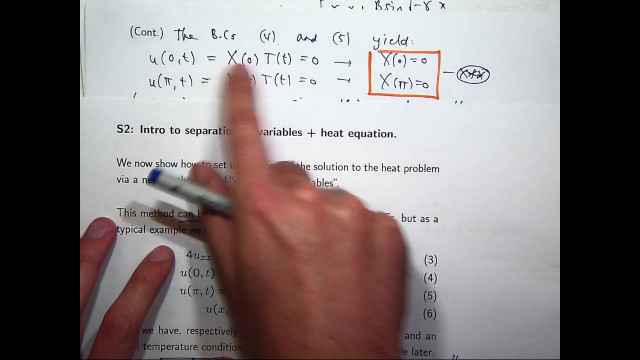 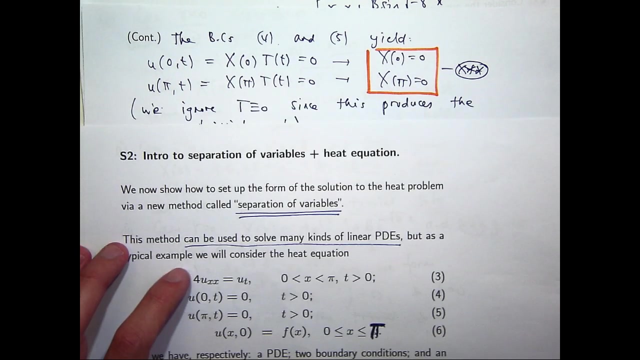 So that's the next step. Alright, So Okay, So Hiding. So the boundary conditions. four and five, together with our assumed form of solution, give us: big X of zero equals zero. Big X of pi equals zero. Now you could argue that. well, what about the case when big T equals zero? 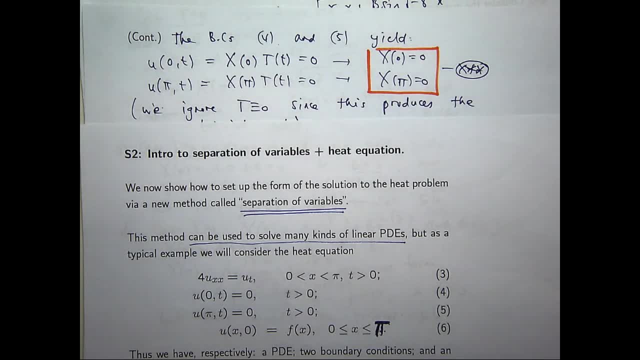 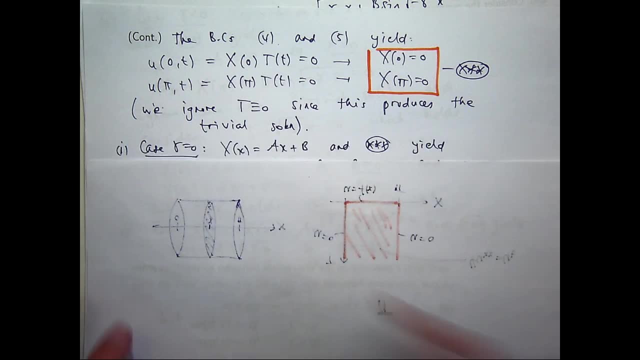 Well, that gives us the zero solution, So we're not interested in that. It's a trivial solution. Okay, So we ignore the case. big T equals zero, Alright, so let's look at the case. gamma equals zero. In this case, big X is this: 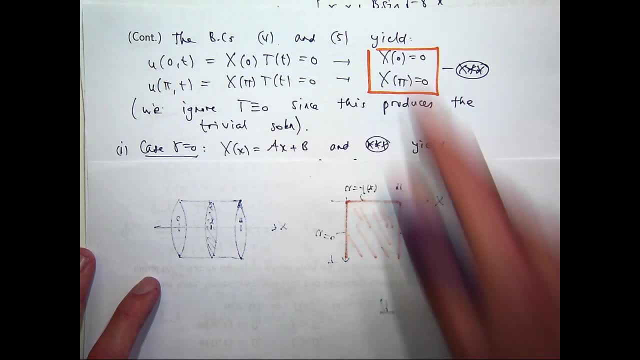 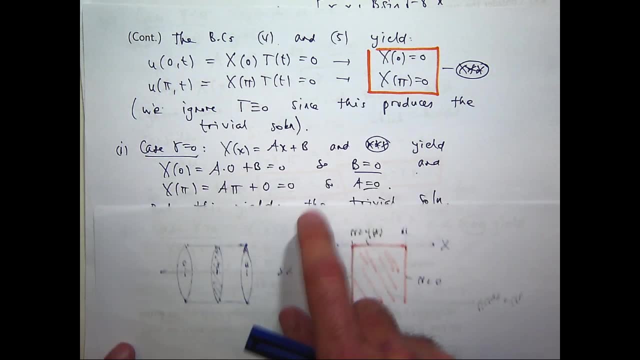 And if you look at this- two boundary conditions- What do you see? Well, The first one gives you B equals zero, And the second one gives you big A equals zero. So if that's our form, and big A and big B are zero, 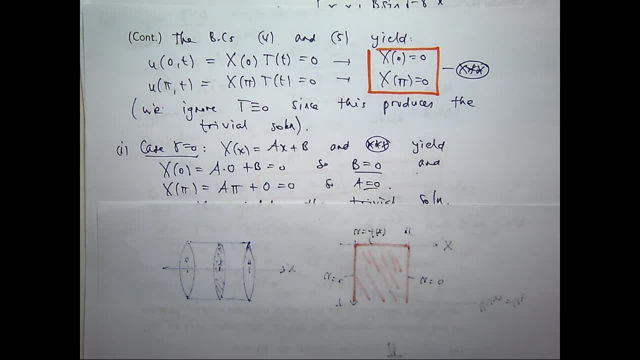 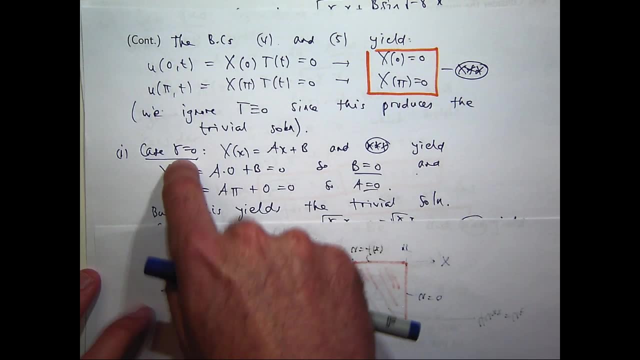 Big X has got to be zero. So again, that gives us the trivial solution. We're not interested in that, Okay, So What this means is that we can ignore the case when the separation constant is zero, So we just forget about it. 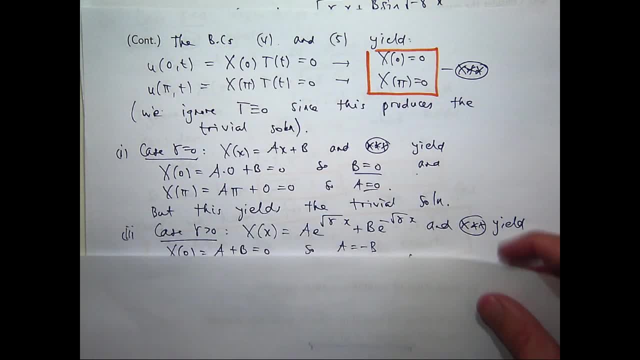 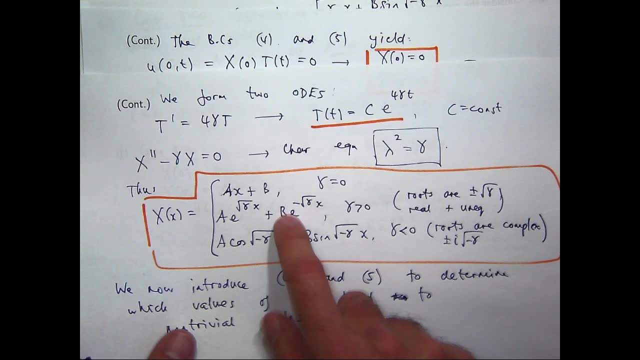 What about the case when gamma equals zero? Well, Okay, So what happens when gamma is positive? Well, when gamma is positive, If we look back to our little chart here, We get a linear combination of exponentials. So let's take this. 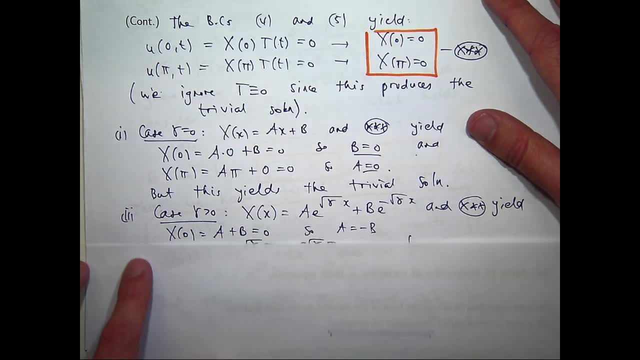 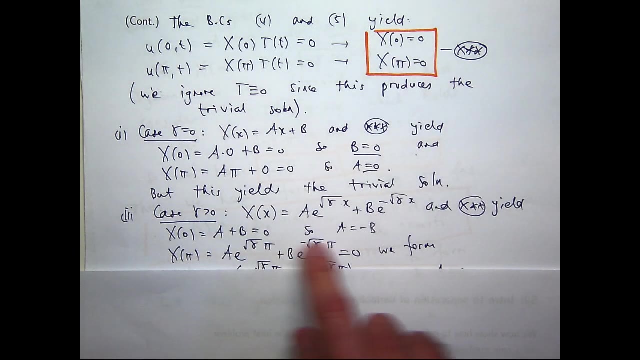 Use these two conditions and see what pans out. Well, the left hand endpoint And the right hand endpoint. Sorry, The left hand endpoint gives us A plus B equals zero, because we just have zero exponents, So A equals minus B. If I sub the right hand endpoint in: 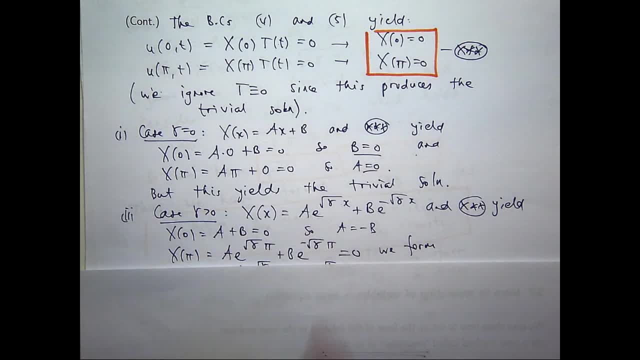 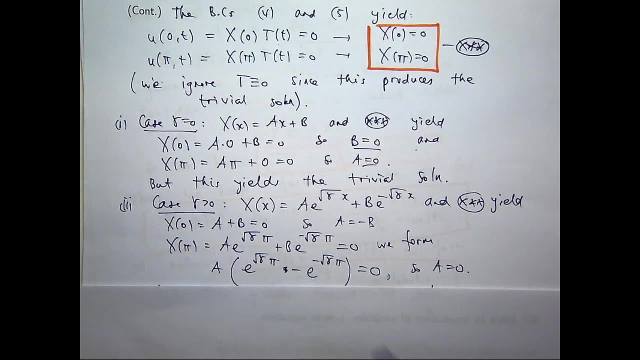 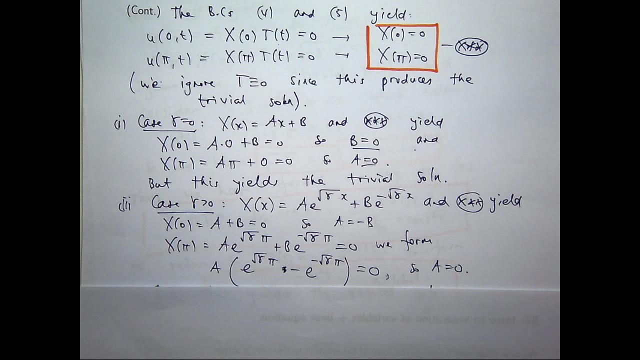 I'll get some equation involving big A and big B. Now, If I put this information into here, I can simplify a little bit and come up with the following. Now, This bottom line, The thing in brackets, can never be zero unless. 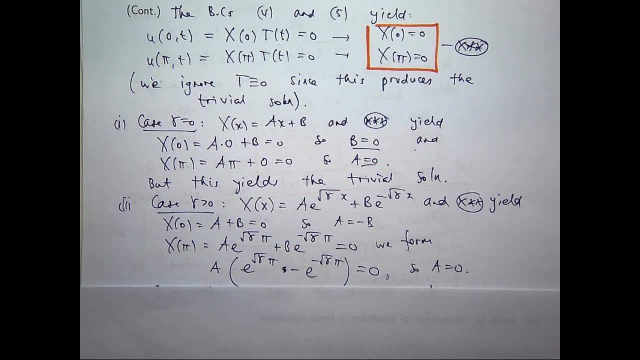 Unless the separation constant, gamma is zero. But gamma is not zero in this case. We're discussing the case when gamma is positive. Okay, So In this context, This thing in the brackets can never be zero. What's the other alternative? 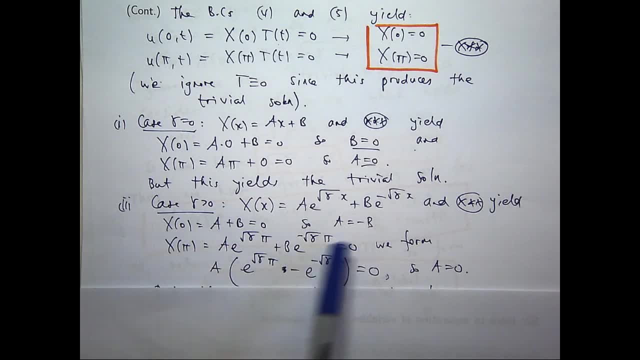 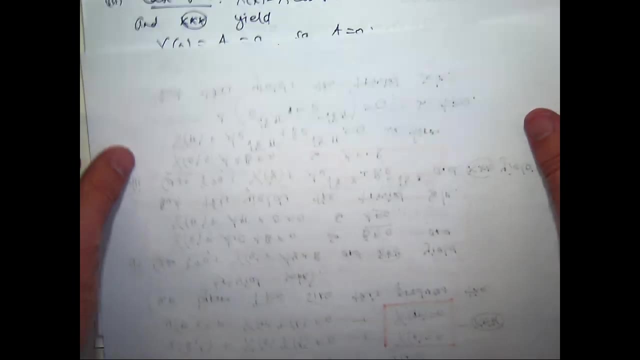 A equals zero. So if A equals zero, B's got to be zero. So what will our solution be? The trivial solution? Not interested in that? Okay, So we've discussed two of our three cases. The last case is When our separation constant is negative. 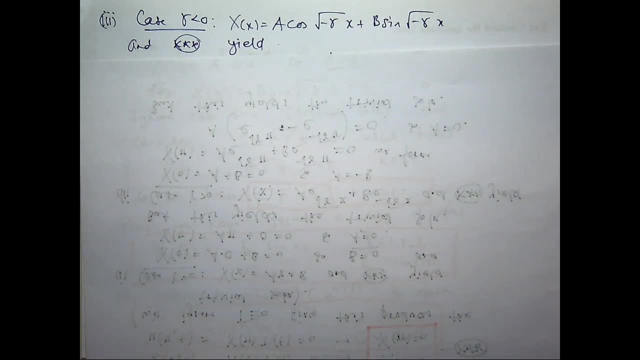 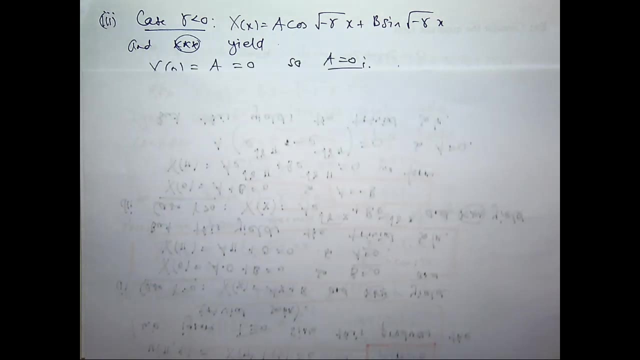 And this is the good case, The non-trivial case. So if you use the boundary conditions again, Then Oh, okay, You get that A equals zero, But the right hand condition Gives us an equation like this. Now One of two things can happen. 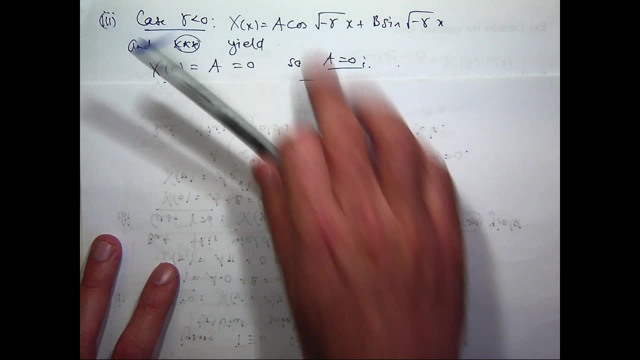 Either big B is zero Or the sign of this is zero. If big B is zero, Then this is zero. The whole thing is zero, Trivial. So forget about that Now. What we're going to do Is we're going to. 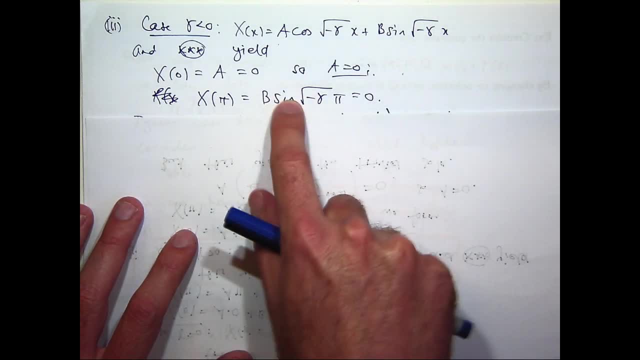 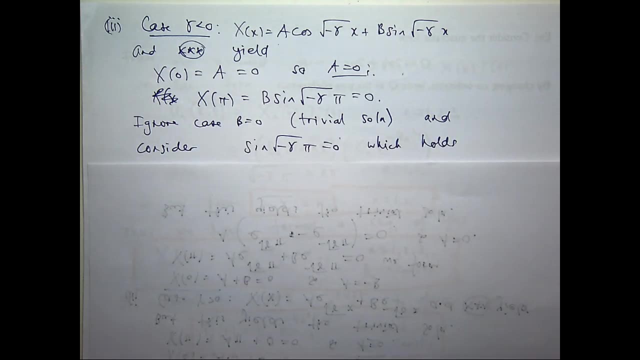 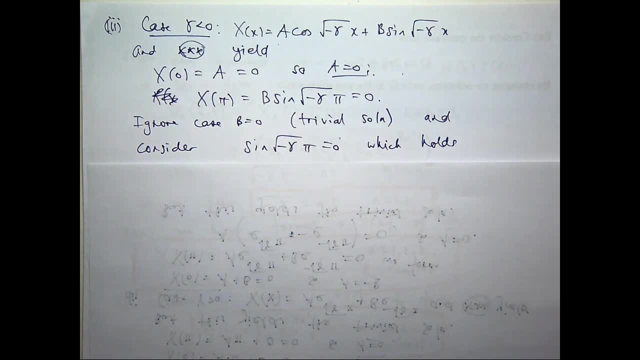 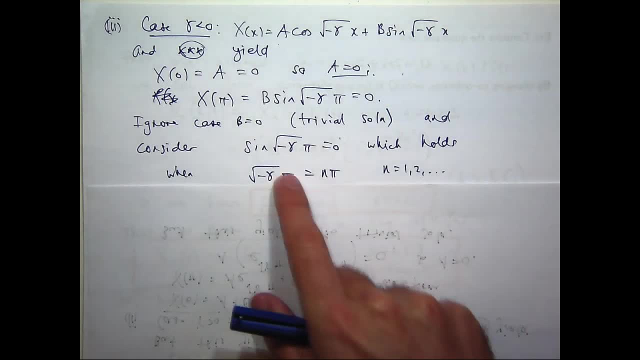 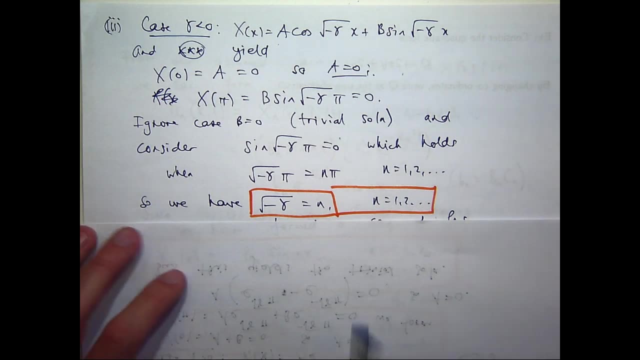 Sorry, Pi Two, pi Three, pi Four, pi Right, So We can form This sort of Sequence Of solutions. Okay, Now you can see the pi's cancel off. So essentially what I have now Is: 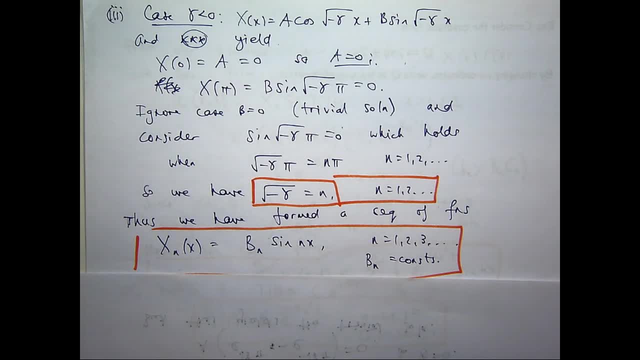 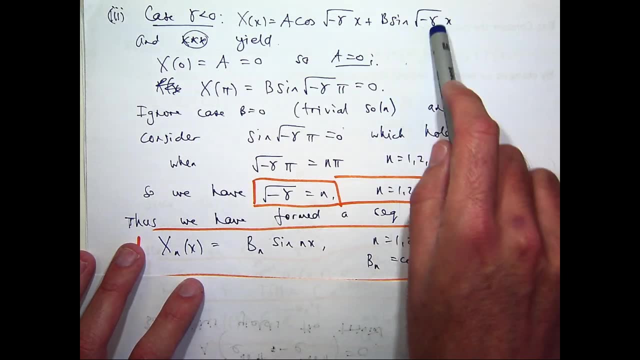 A sequence Of functions. Okay, So all I've done Is I've gone up here. Big A is zero And I've replaced Minus root gamma With n, And because This is A function of interest For 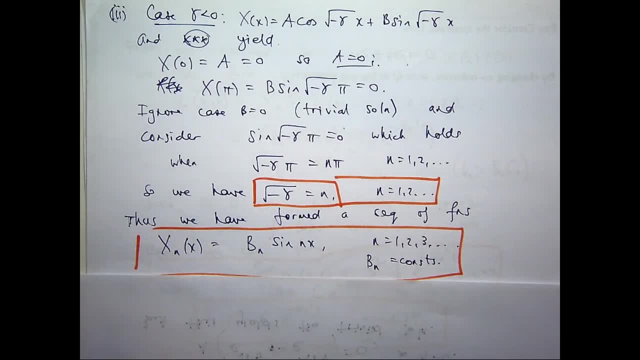 Each n, I need a special constant For each n. That's why the b sub n's there. So Because I need a constant B sub one, B sub two, B sub three. Okay, So now In, Just out of this process. 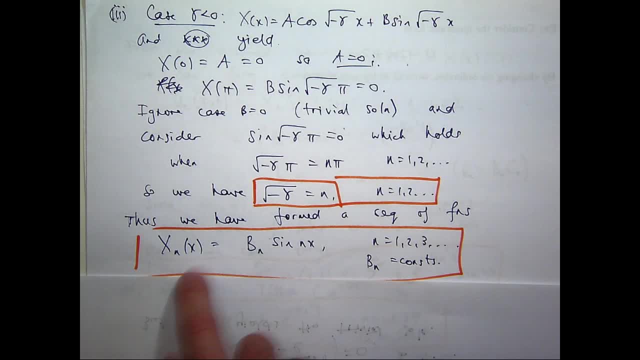 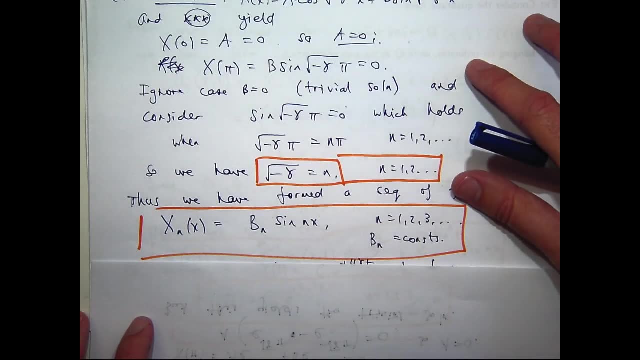 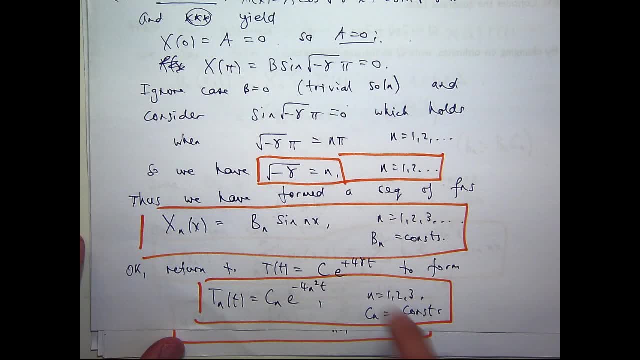 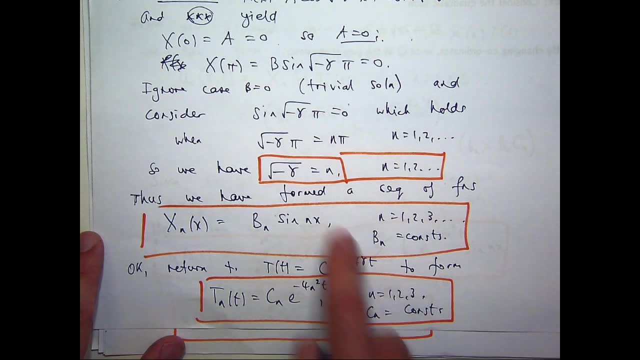 To this Um Equation That we Had on previous pages, And just Let's just Replace Um. We can square both sides, And So we'll get Minus gamma Equals N squared, And then take the minus sign. 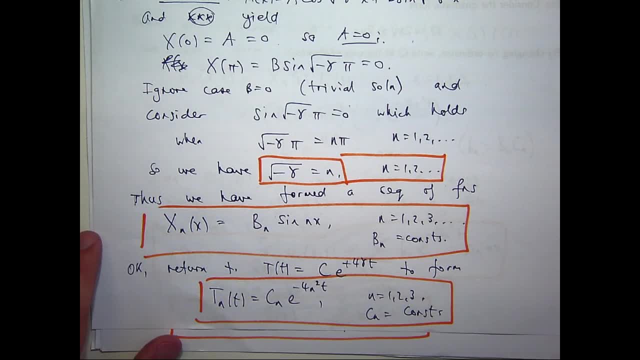 To the other side And replace gamma With minus n squared. So again I can form A sequence Of functions. So the c sub n's Are a sequence Of constants Here. So let's take these two forms. 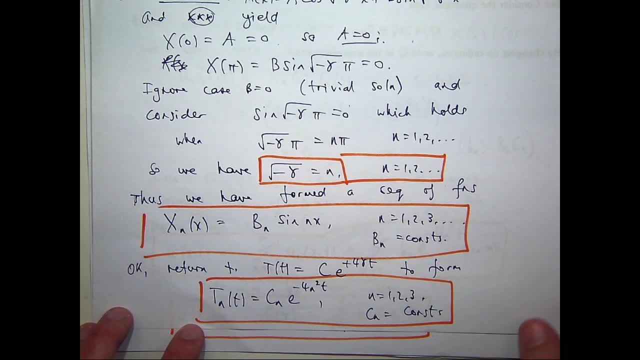 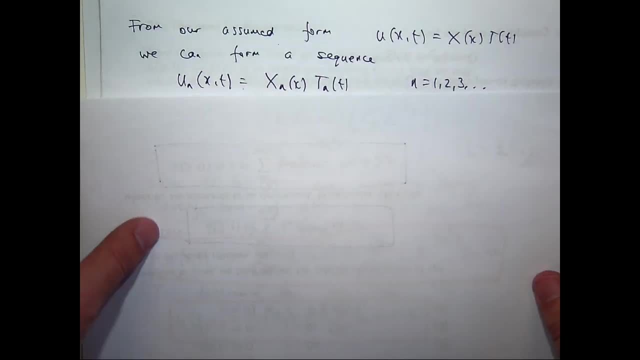 Multiply them together. Okay, So this form's- Um, Uh, Slightly, Uh, Changed Now To this form. I've now got a sequence Of functions Of interest. Okay, So now I've got A sequence. 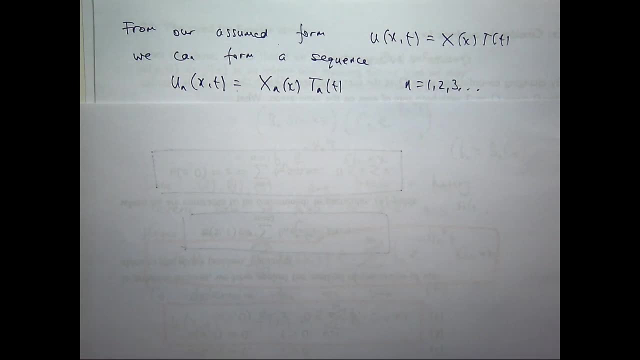 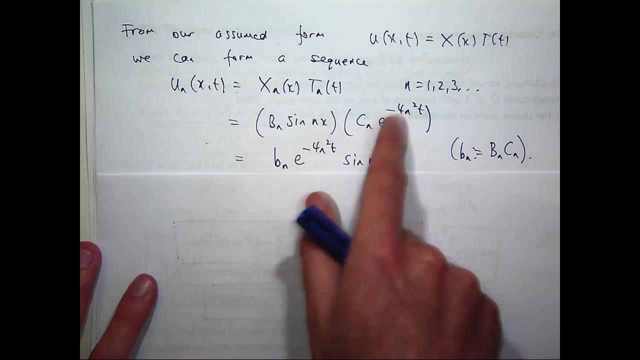 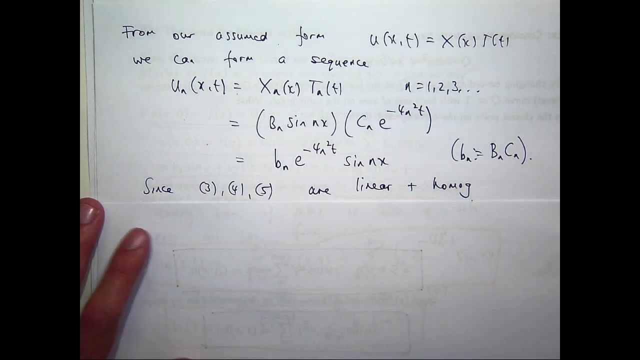 Of functions Of interest. Okay, So I've got A sequence Of functions. Okay, Now Because Our PDE? Okay, So Just Writing those out And just making this sort of Simplification. 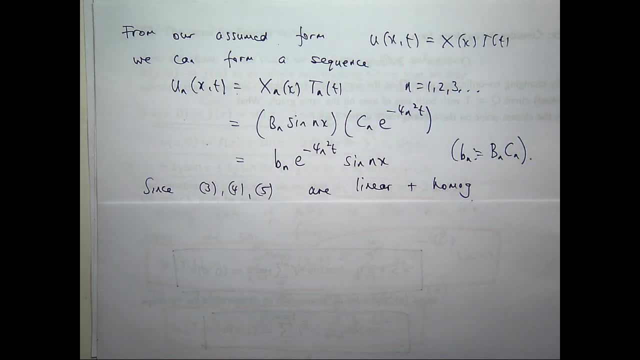 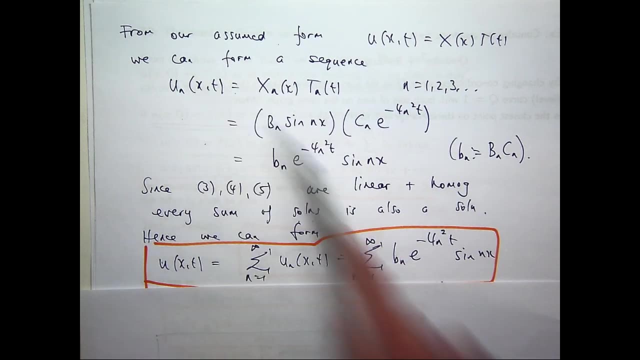 Since our PDE And These boundary conditions Are linear And homogeneous, Then We can use A superposition rule. It says that If I've got all these, This sequence Of solutions here, Their sum. 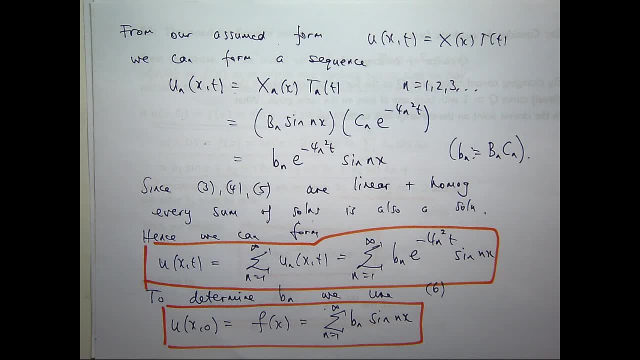 Is also A solution, My sequence Of functions, Sequence Of solutions, And form An infinite sum. There's an infinite value, Number Of n, here, So I need to form An infinite sum. Now The last thing. 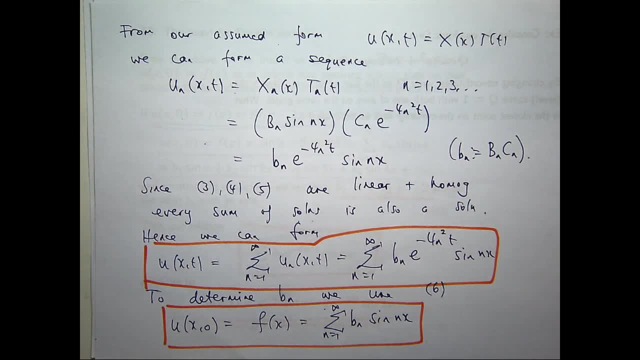 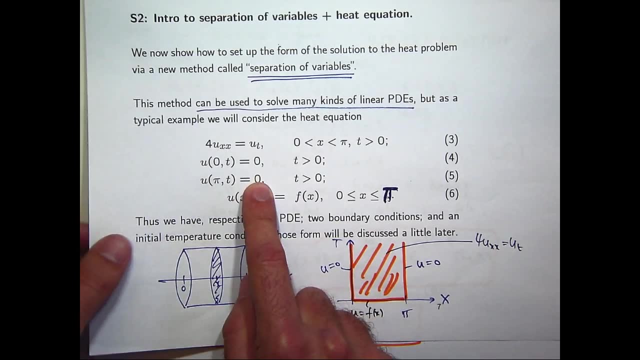 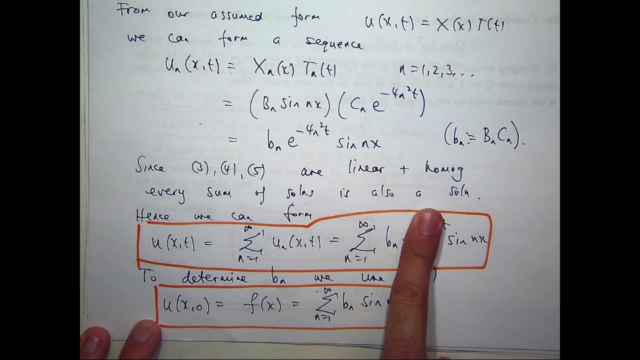 That we Haven't used Yet Was The Initial Temperature Function. Okay, We haven't used That information. We've used That, That And that T equals zero. Well, The exponential Will just become one. 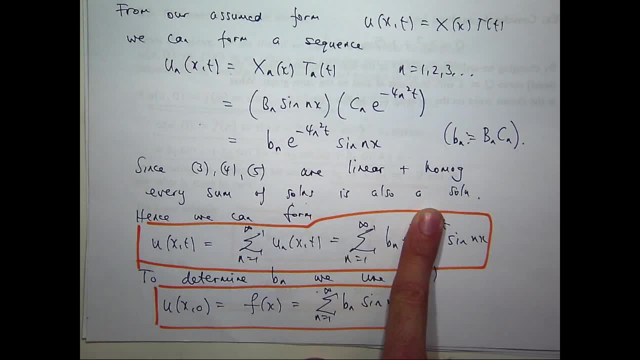 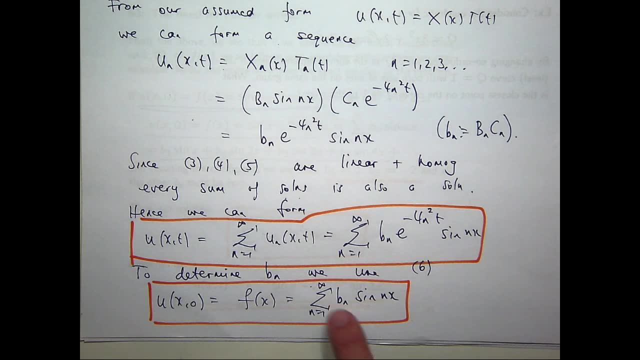 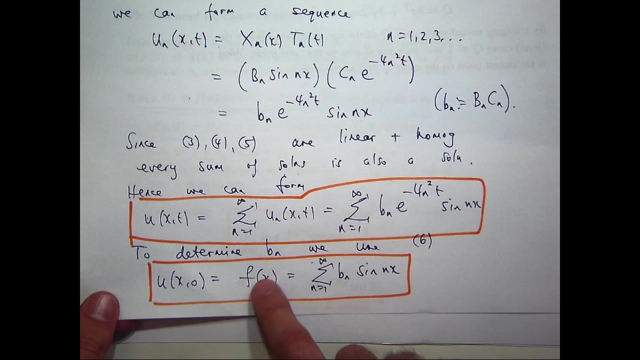 And I can Just Write down My f of x And my series. So The question Was: How Do You Calculate The Psi Bends From This Relationship? Okay, Well, 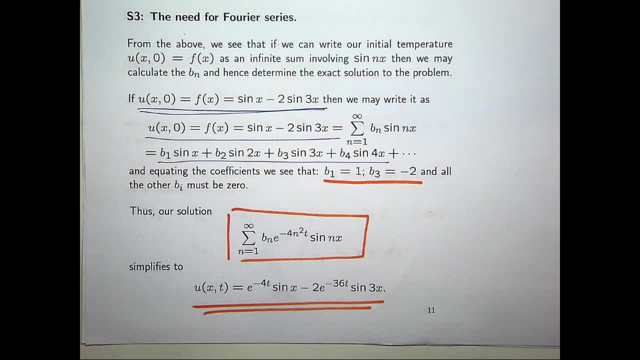 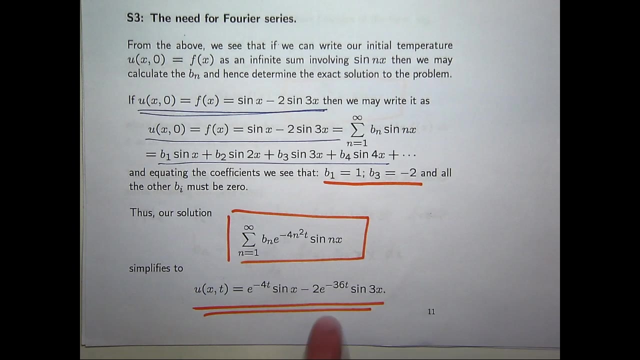 It Depends On The Finite Sum Involving Sine X, Sine Two X, Sine Three X, Et cetera. Right, Then, You Can Just Equate. 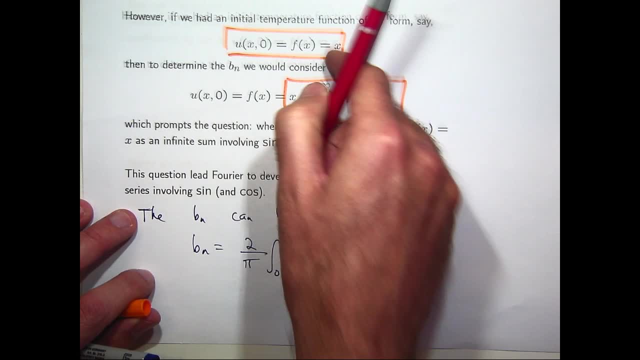 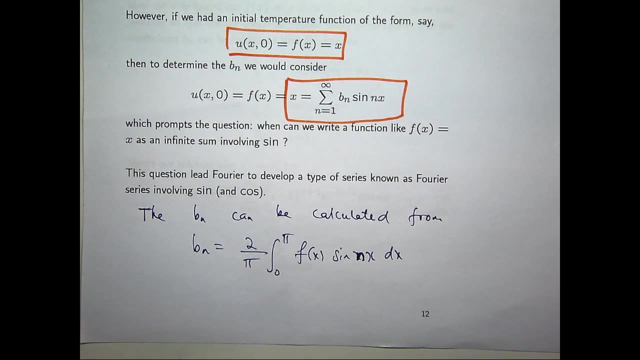 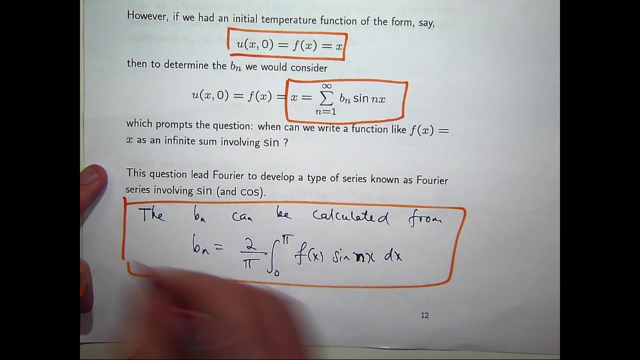 The Coefficient And Come Up With A Solution. Fourier Series Is In Terms Of This Fourier Sine Series And Calculate The B Sub Ends. Okay. 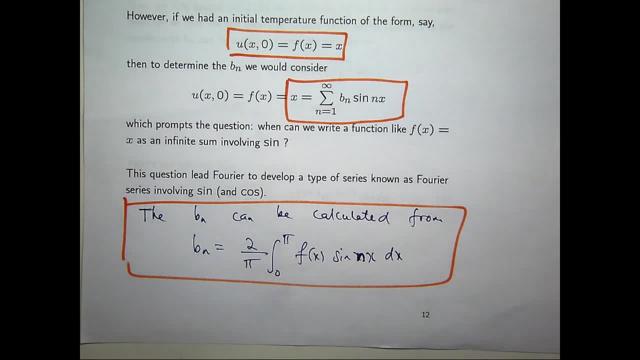 Well, I Claimed That This Is, This Is What, How You Can Actually Calculate The Functions. I Would Extend That Temperature Function As An Odd. 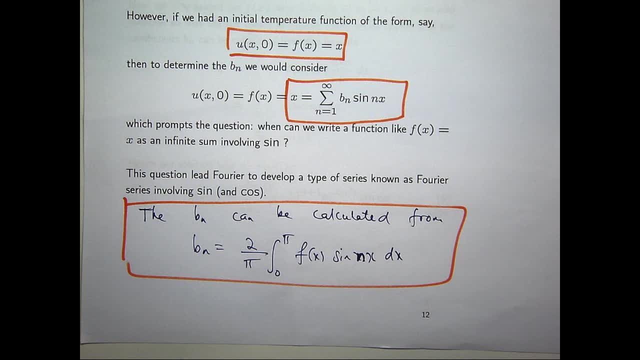 Function And, If I Wanted To, I Can Make It Periodic So I Can Extend The Temperature Function Outside Is Continuous, Has A Piecewise Continuous. 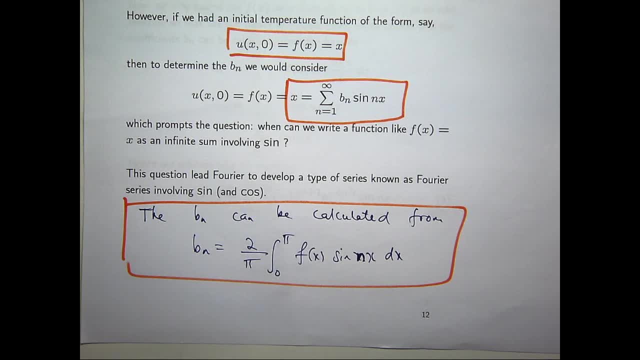 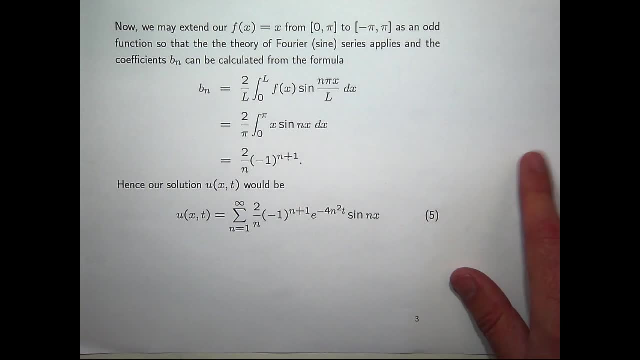 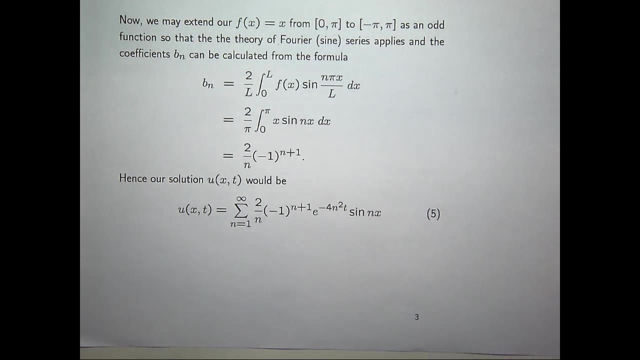 Derivative, I Can Form The B Sub Ends From This Formula. Okay, So So Now. So This Is Now On The, On The Latest, So. 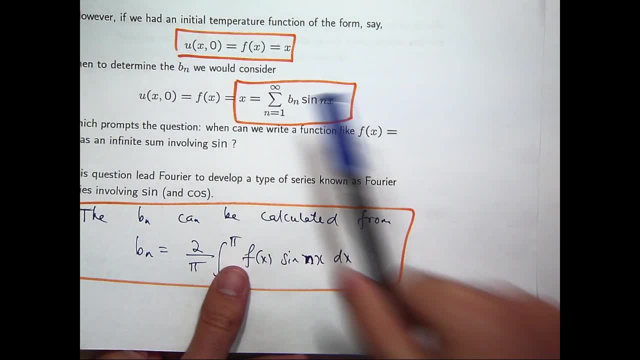 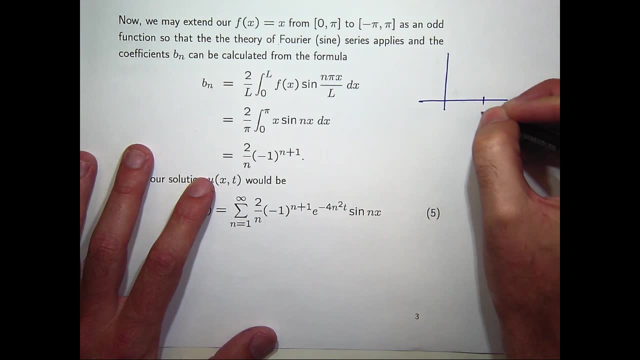 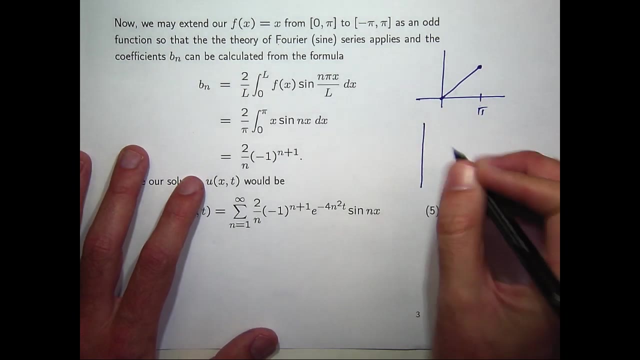 I'm Faced With This. I Can Extend My Temperature Function As An Odd Function. So Initially Let's Just Go Here. Okay, I Can Extend. 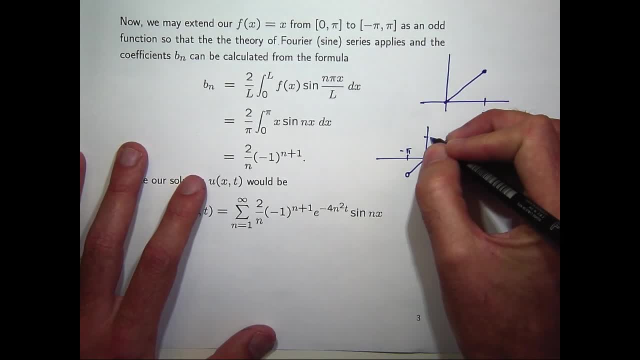 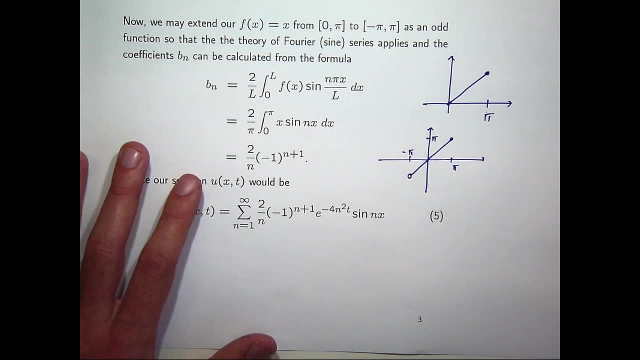 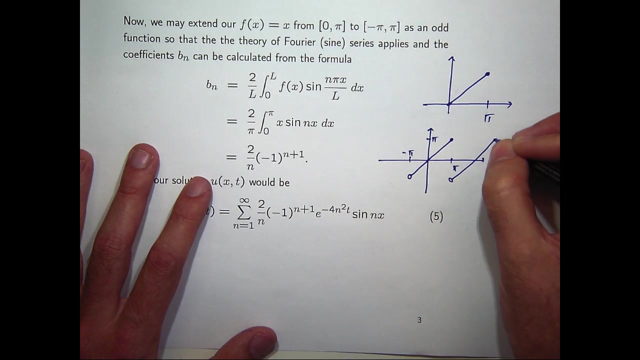 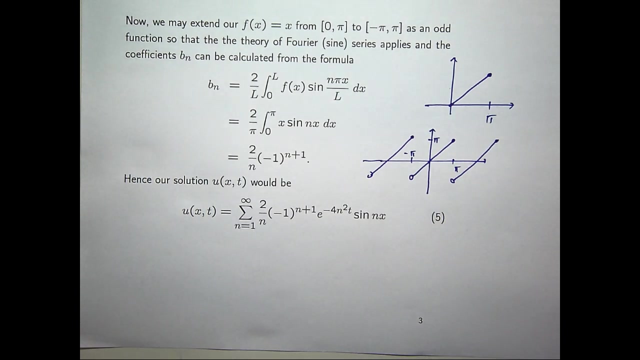 My Function As An Periodic Function. Now I Can Also Extend It As, Say, A Periodic Function. Now That Function Is Piece, Wise, Continuous And 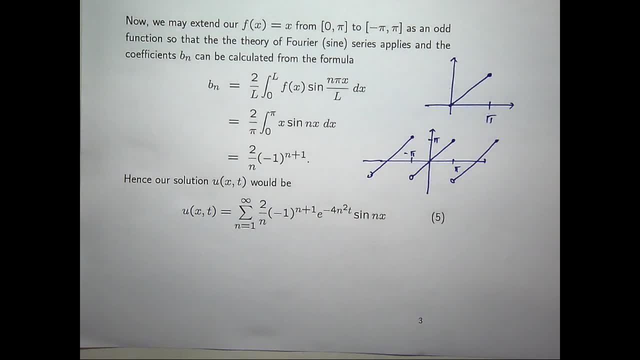 It Does Have A Piece Wise Continuous Derivative, So I've Got No Problem Calculating The Fourier Series. Okay, So How Do I Actually Calculate? 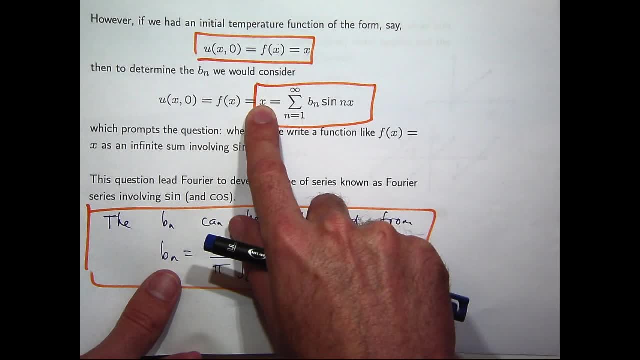 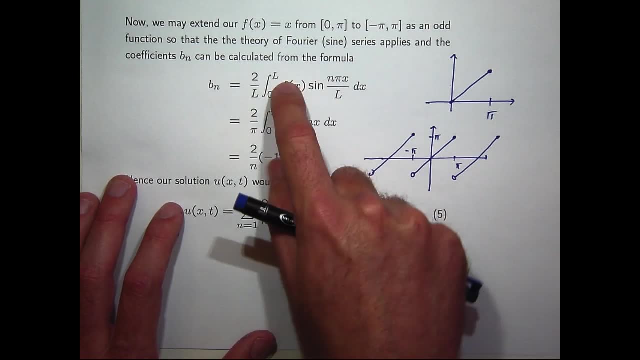 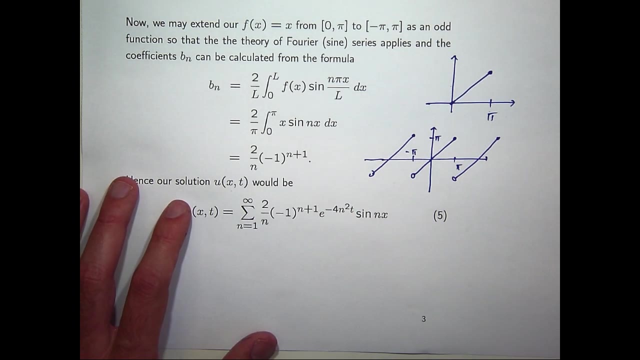 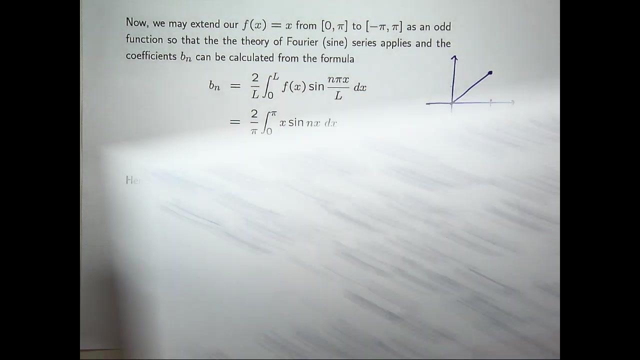 The The Fourier Series. Well, I Want The Fourier Sign Series. Okay, Comes Back To My General Form. Yeah, And Just Replace B Sub In With.